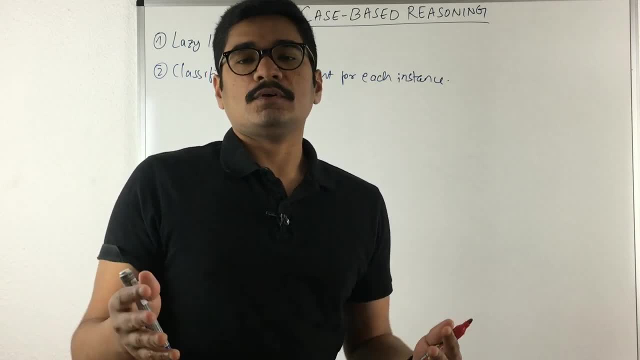 manner. So you have a kind of recognize spaces in case of KN nearest neighbors. So that is another property and third properties that Att notation is given to that same system and then it will callіт a specific newer倡 to And third properties that these instances are labeled. GP wrote Long've that they are lazy learners, that is a chamfer of the Klein aliases or that create a Middle- surfers demonstration. 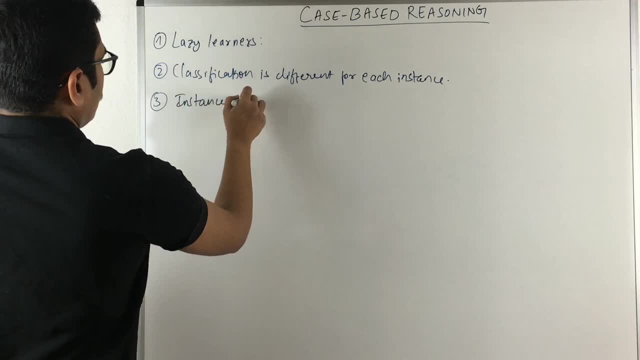 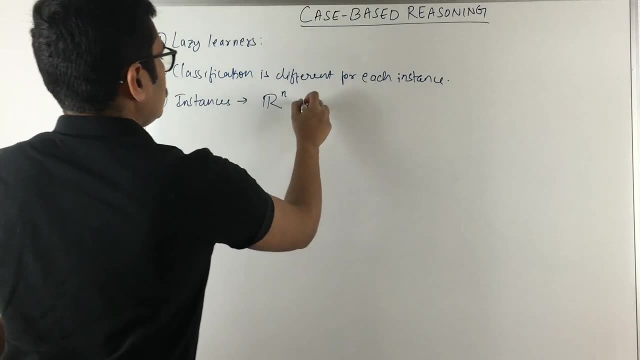 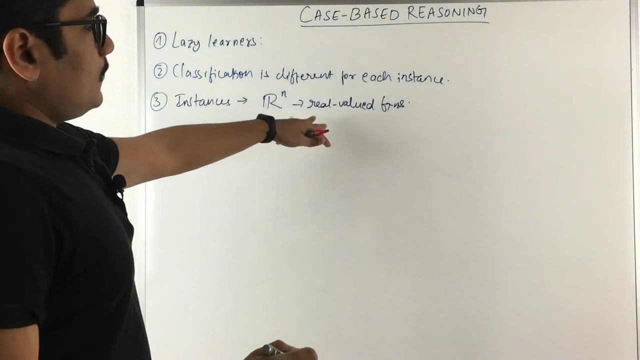 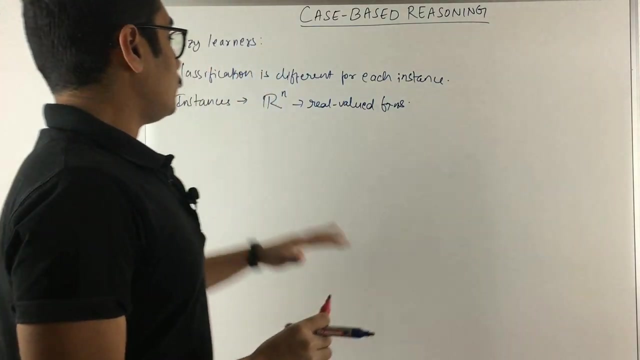 cases And instance And that these the are represented in n-dimensional Euclidean space. So these are basically real valued functions. So mainly they work upon real valued or discrete valued, but, especially since we have taken the case of k nearest neighbors, they will mainly work upon this real valued. 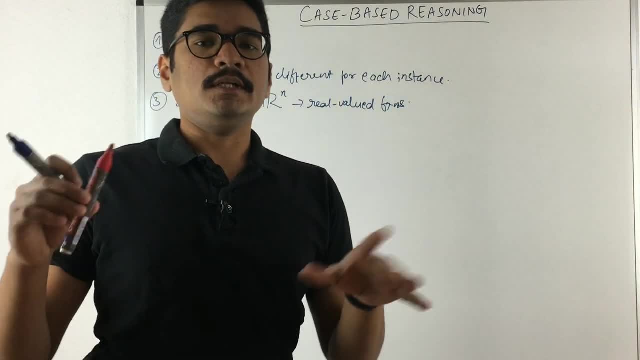 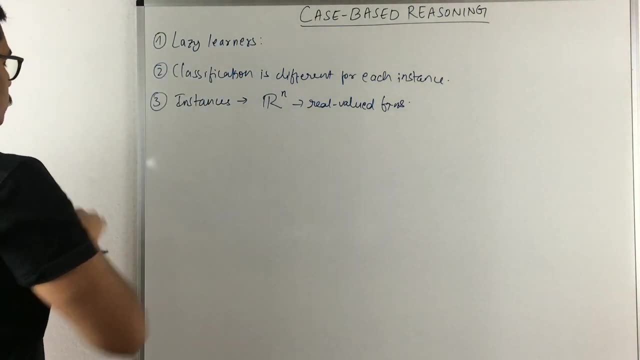 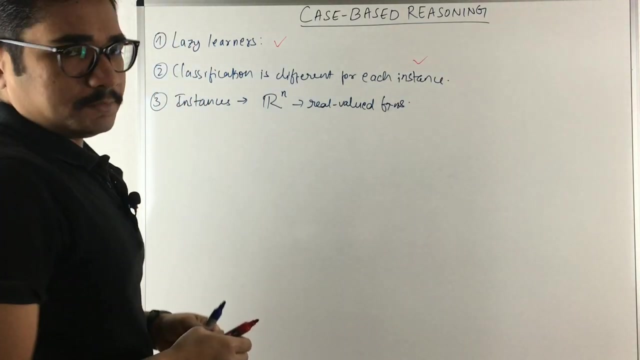 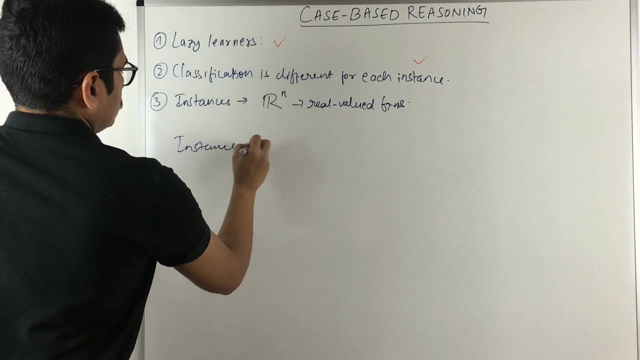 function, since in k nearest neighbors, we have to deal with all the neighboring points which are in r-dimensional Euclidean space. now, case based reasoning systems works on the first one as well as the second one. now why these two properties are based on case based learning? because the instances in CBR are symbolic representations. 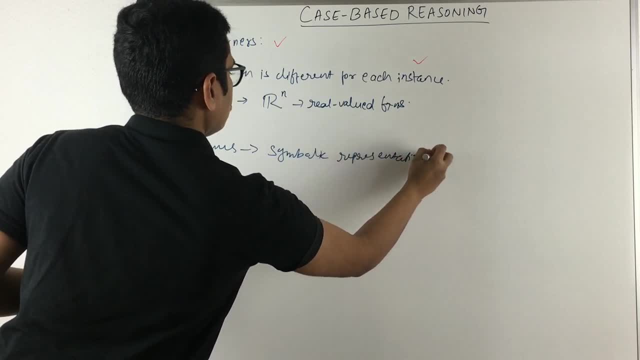 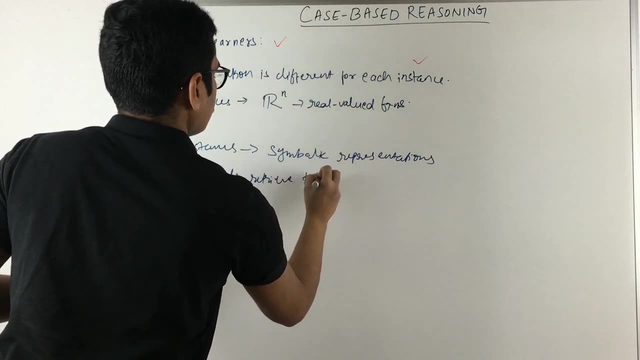 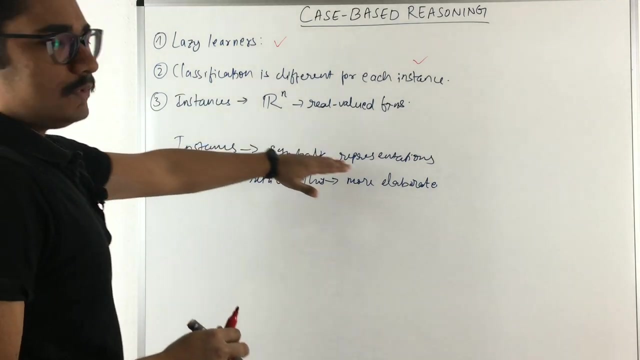 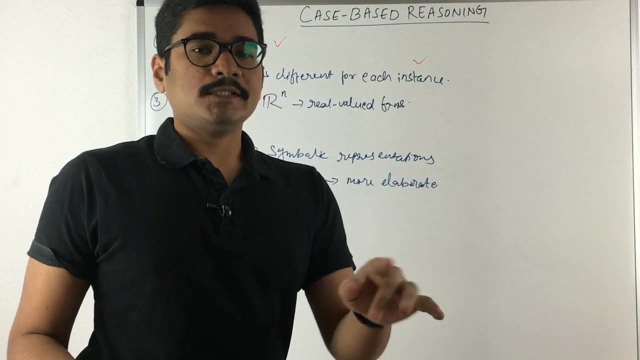 So So, and the methods which are used to retrieve this are more elaborate. Let's get into this detail a bit later. So, basically, you don't have any real valued or any continuous valued numbers in order to represent case based systems. So, basically, each and every instance is considered as a unique, different case. 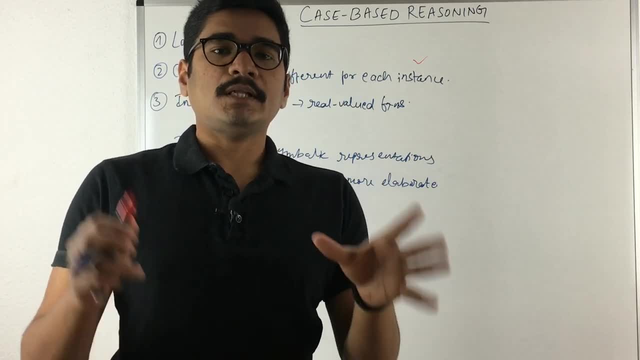 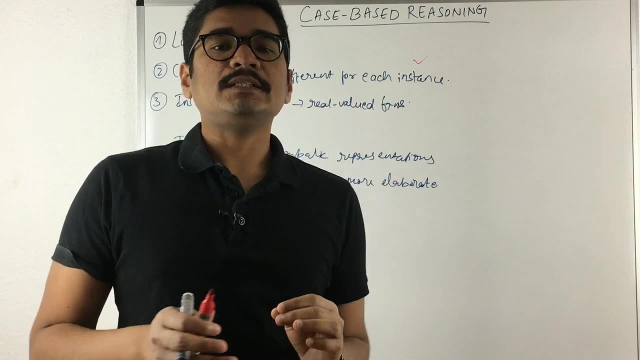 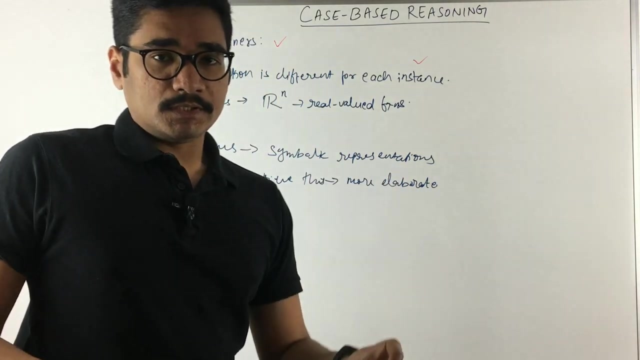 Say, if you want To provide a loan to particular customer, then that particular customer is considered as a case and then, based upon the previous use case scenarios regarding that customer, it will propose a solution. So, similarly, you have symbolic representations for each and every instance and you have methods. 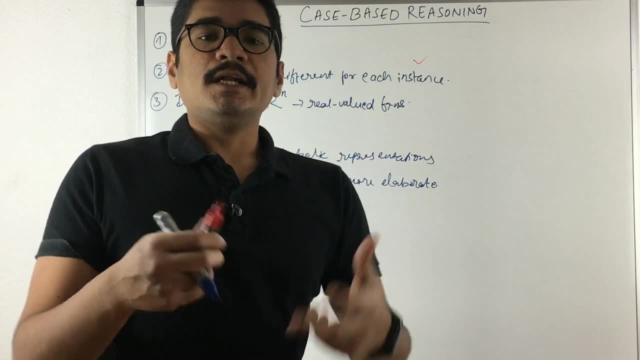 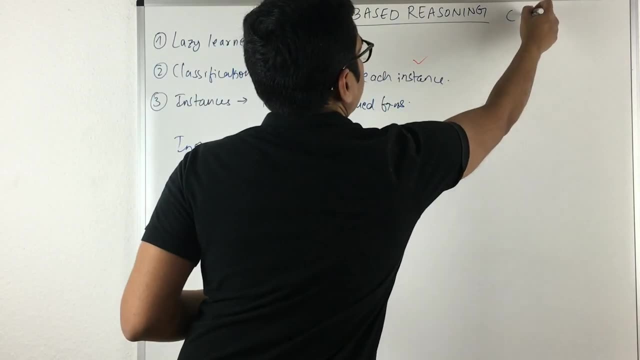 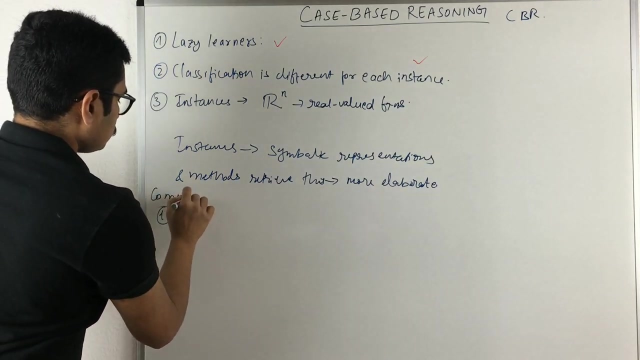 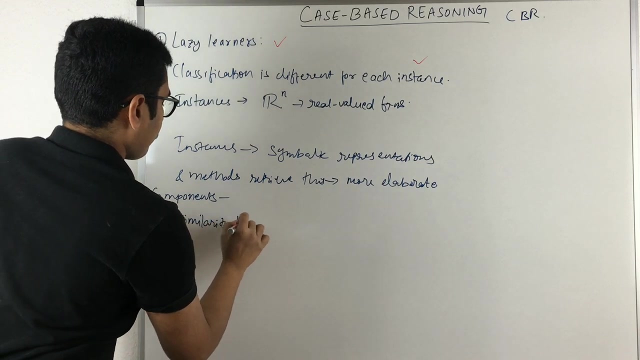 that retrieve and which are more elaborate regarding the functionality of that particular use case system. Now, this case based systems, That is, this CBR, has got three different components. So first component is: you need to have a similarity function, our especially a distance measure, in order to 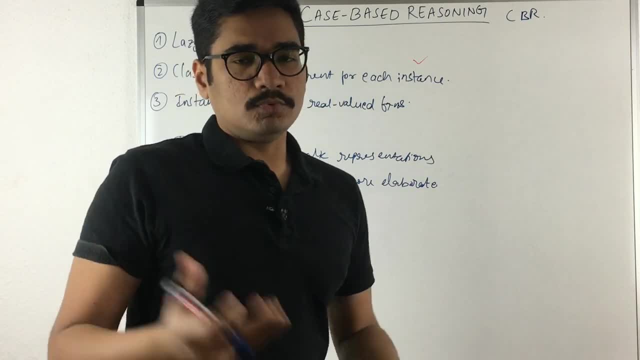 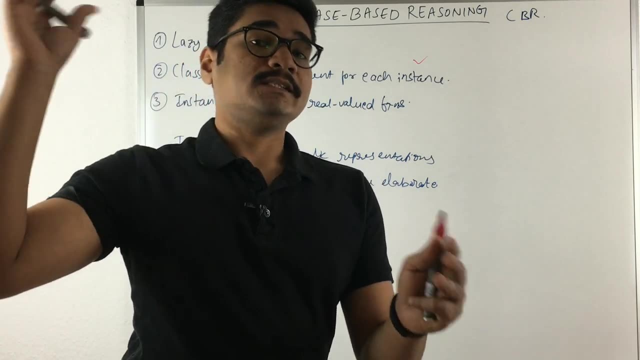 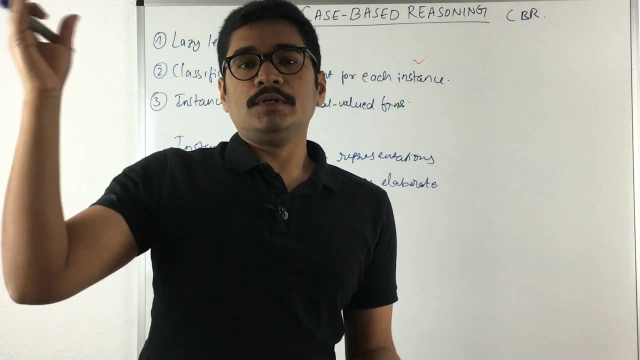 measure the similarity among the instances. so, given a problem to your case based reasoning system, It will approximately try to fit a new solution. but it's not the exact solution that is stored before, so there can be similar kind of use cases in the before-past history. 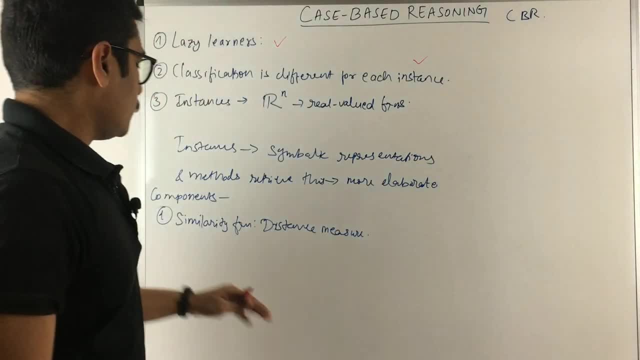 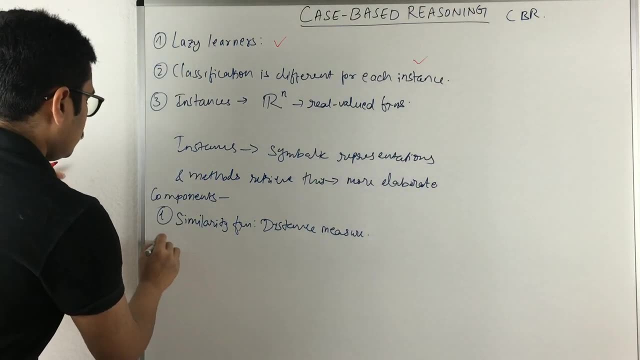 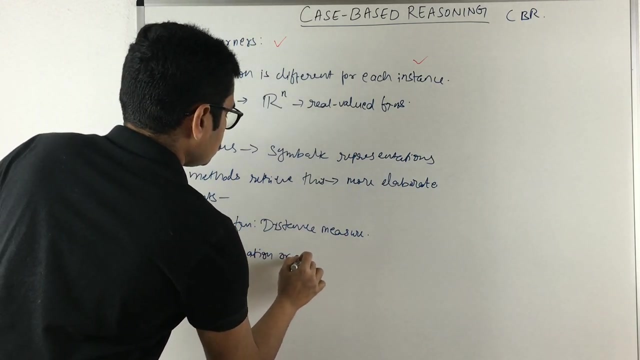 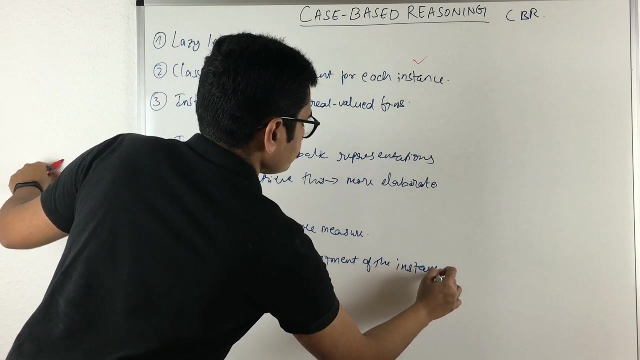 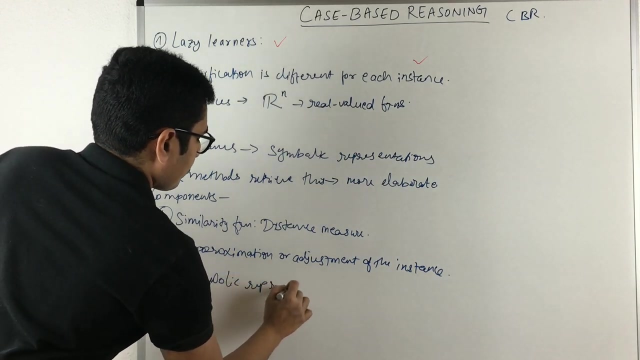 So it will try to suggest some new solutions based upon that. So for that you need to have some similarity functions, So we mainly use Euclidean distance in that. and second, you need to have some approximation or adjustment of the instance. and third is that you need to have symbolic representation. 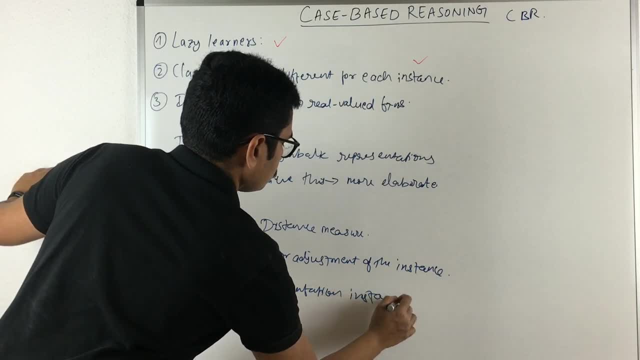 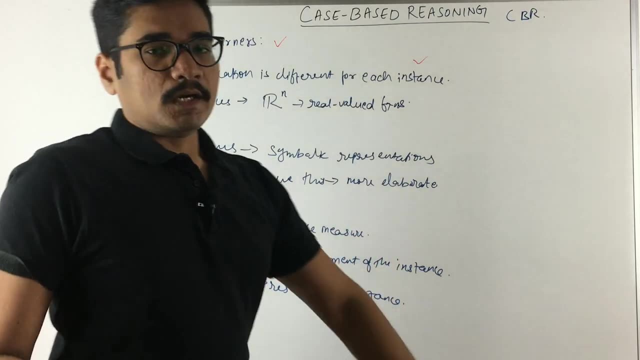 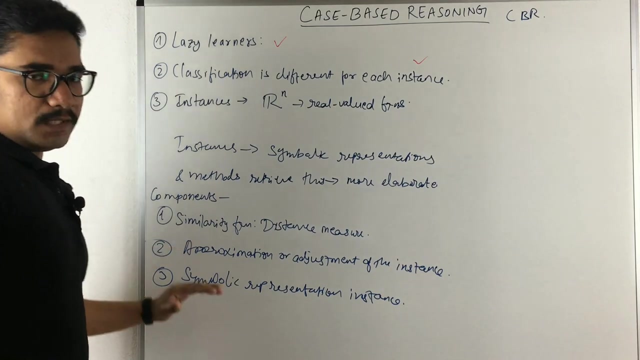 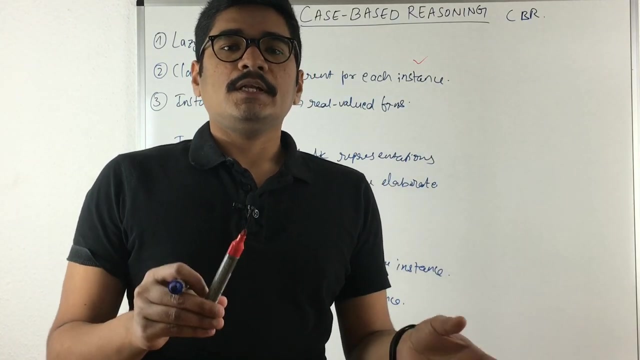 of the instance. So when you are proposing a particular solution, you need to have some approximate kind of representation in order to show that or in order Display that. so these are the basic three components on which CBR systems work. So whenever, for a case-based reasoning system, you give a problem, then it will try to derive. 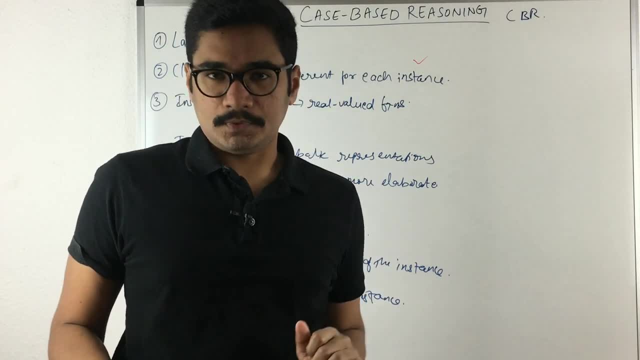 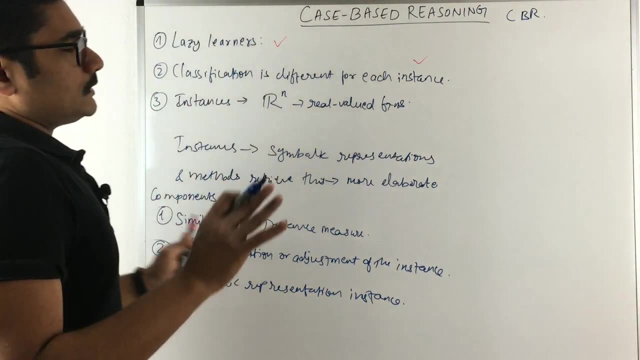 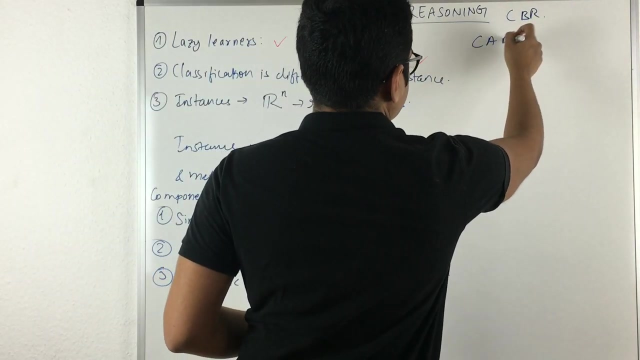 a solution based upon the solutions of the previously stored problems. So that is an important property which is seen in case-based reasoning systems. So now we just take a scenario based upon all these things We have spoken, say we are having a cadet system. 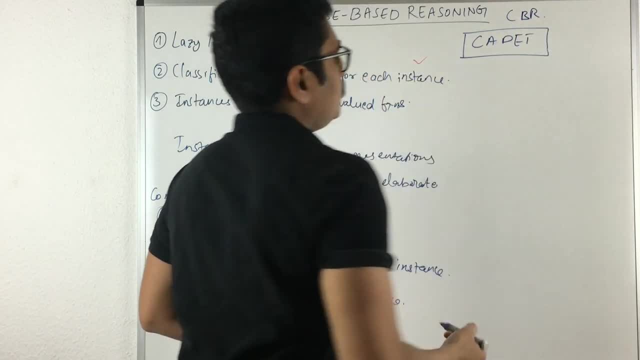 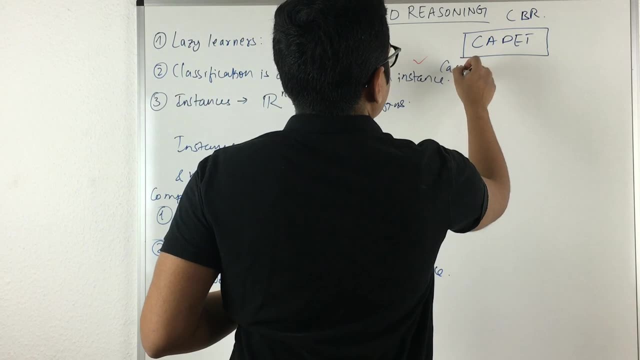 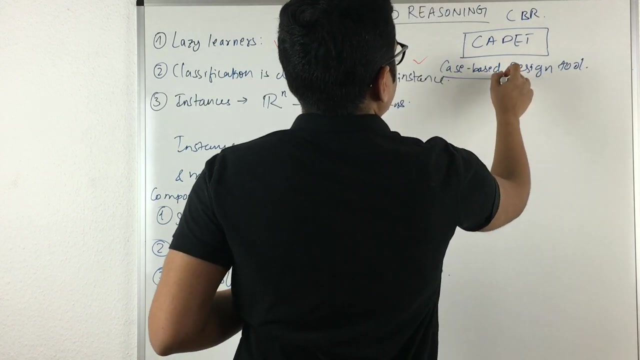 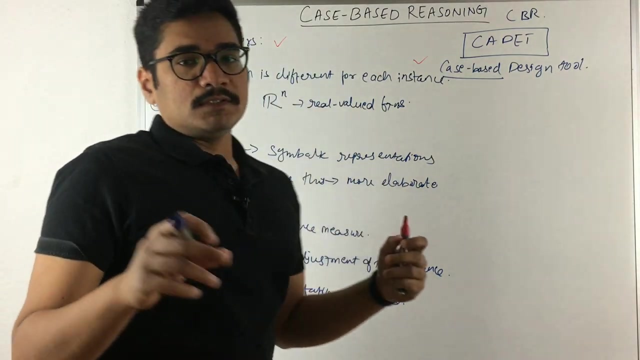 So for modeling this case-based reasoning, what you mainly use, a cadet system. So cadet stands for case-based design tool. that is, case-based design tool. This case-based is for CA design and tool. So now what we have is we need to design water faucets. 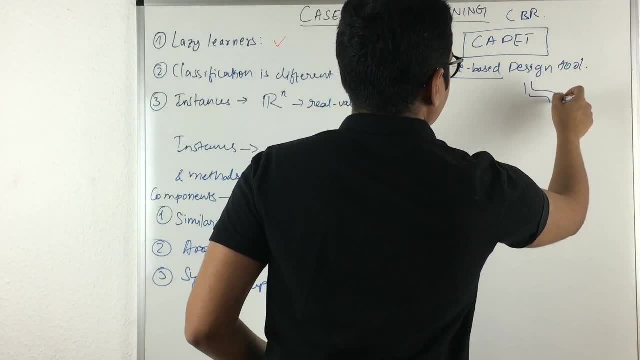 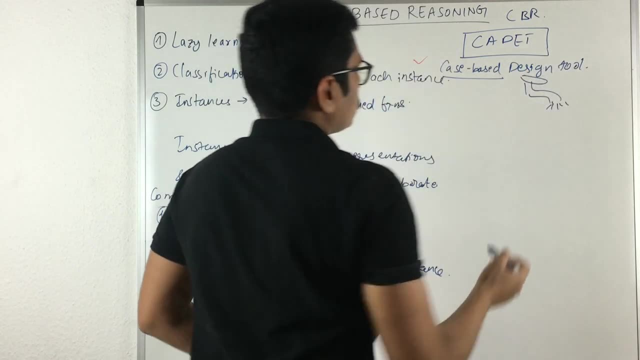 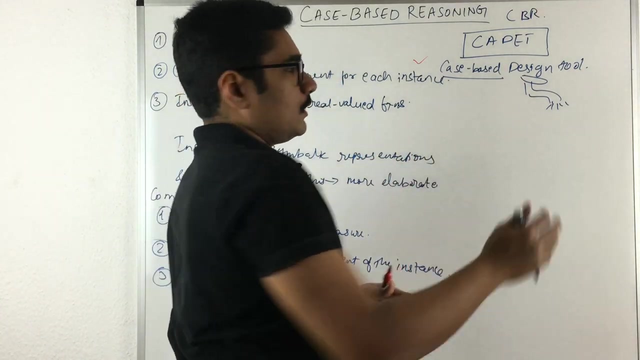 So water faucets are basically your water taps. So where in the modern water taps what you basically have is you have a lever, something like this: So you basically just shift this to the left side for a cold water, or you should this to that side- right side- for the hot water. 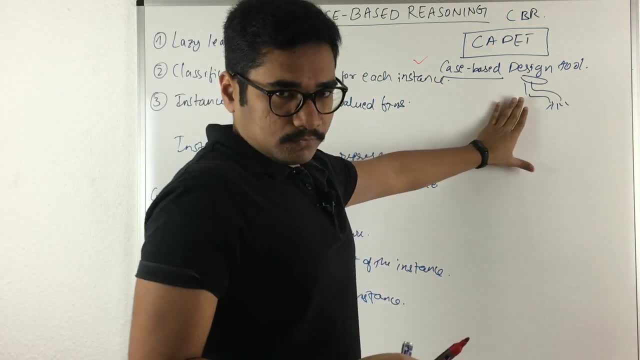 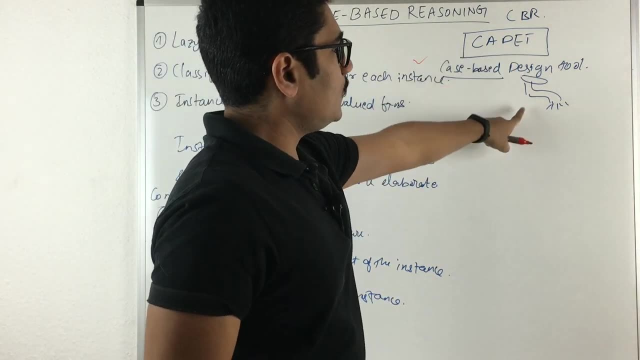 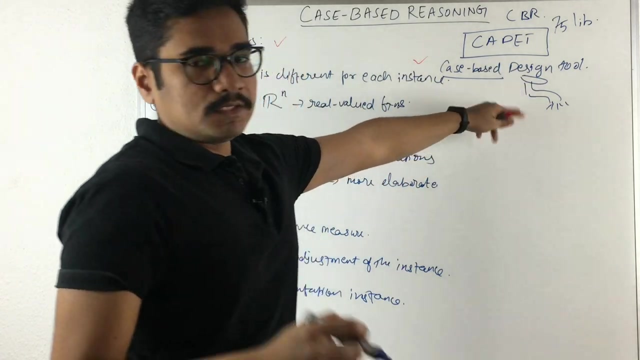 So, similarly, we have to design water faucet by using the case-based reasoning system. So what I have is for this cadet system. if I want to build a water faucet, something like this, It has an inbuilt 75 libraries of previously stored frameworks of this particular kind. 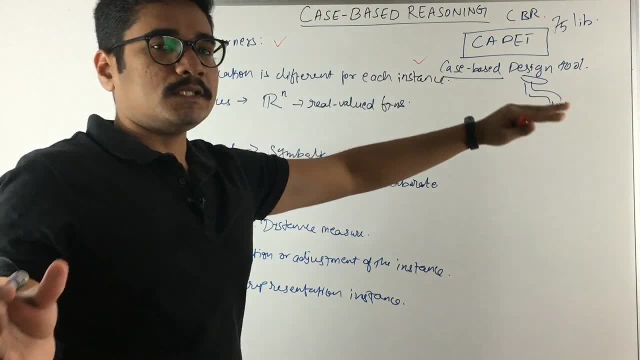 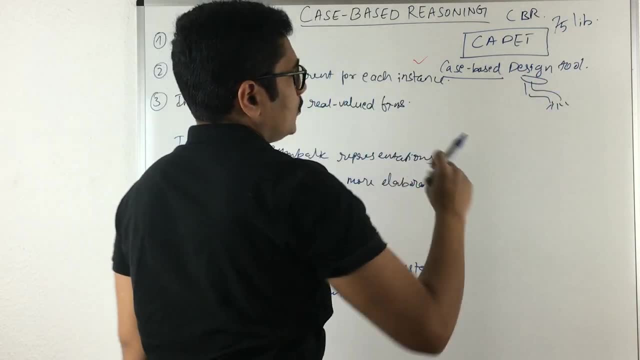 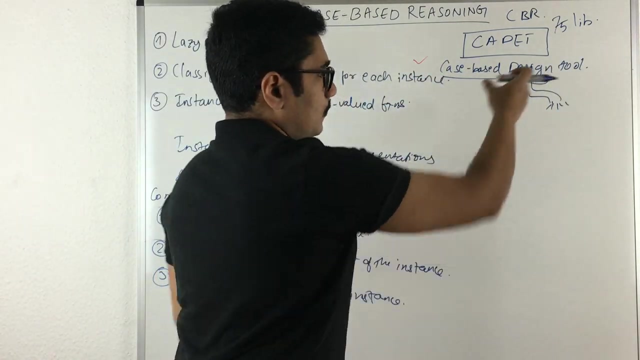 of structure or something like that which is there in plumbing scenarios or like that. So what I have is so, out of this 75 libraries, I am taking the most representative or the one which has more similarity to this use case problem. So, according to my euclidean distance, 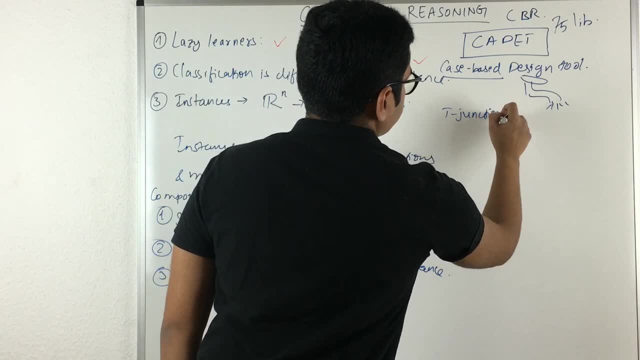 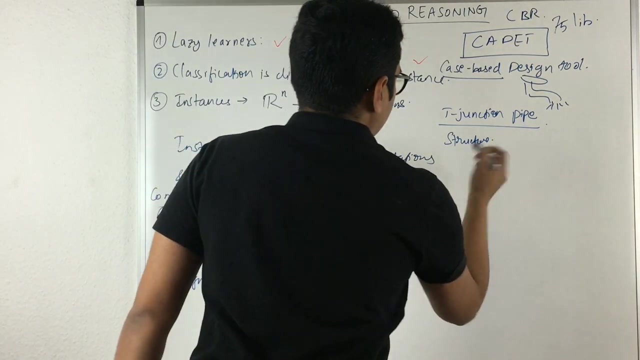 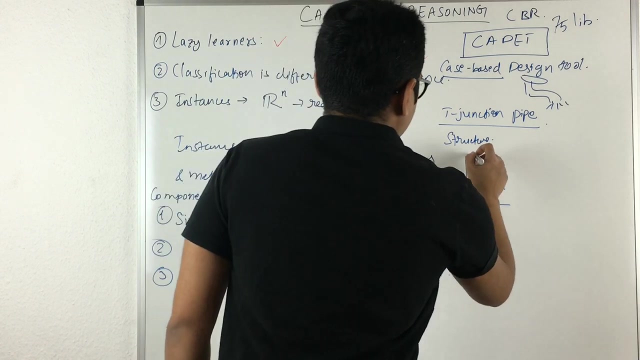 I called as a t-junction pipe, So I have a t-junction pipe. So first, basically, you need to have the symbolic structure. So instances in CBR are represented by using the symbolic notation. So in symbolically what I have is I have a system like this. So say I have from here. 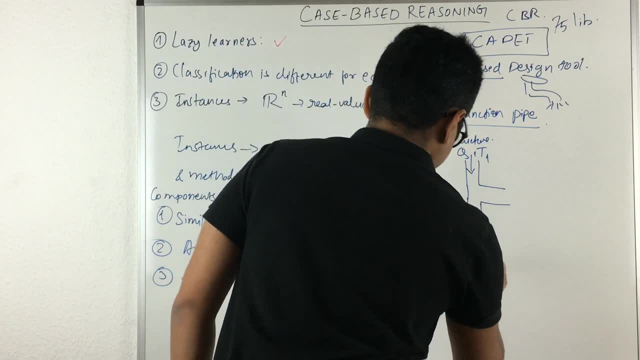 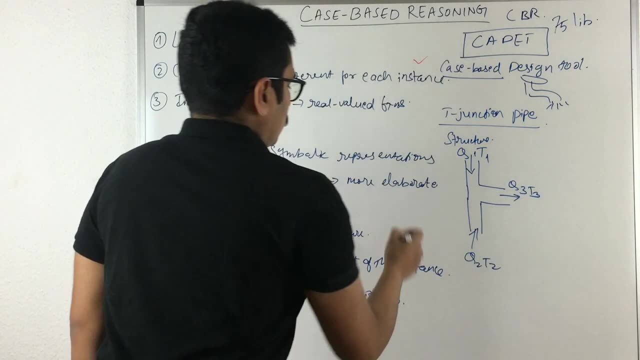 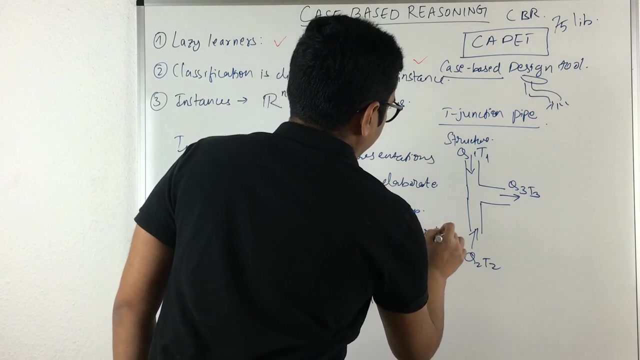 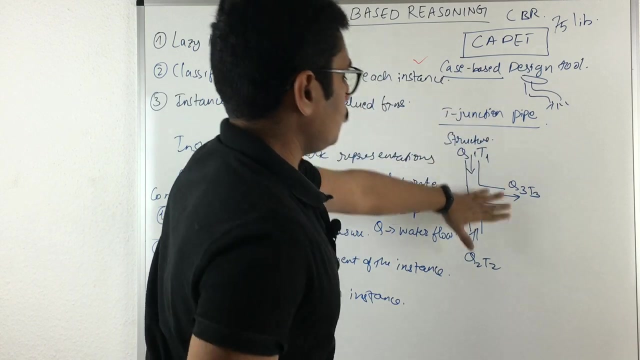 q1, T 1, q 2, t 2, and say, here I have q 3, t 3. now here T represents for the temperature and Q represents the water flow. So Assume, like this is a t junction pipe and you have water. So if you want Cold Water, what we basically do is you just open this. 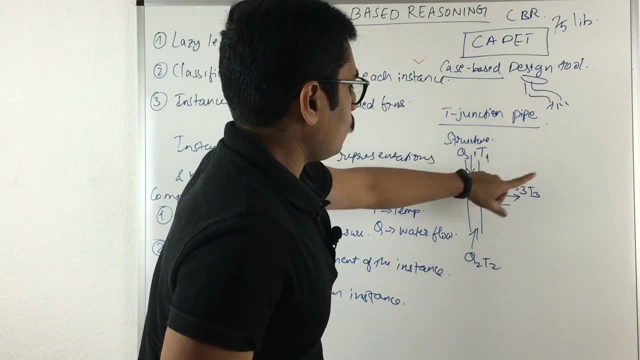 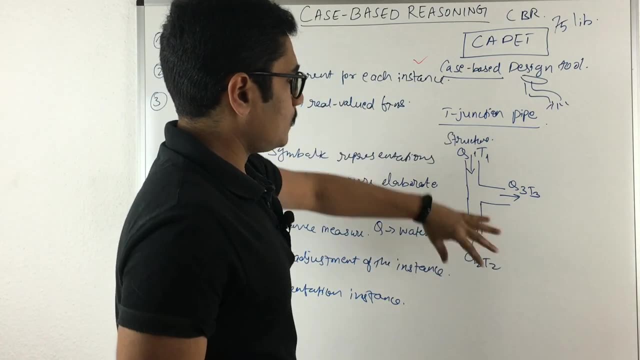 tap and prevents a water flow going again and you keep it closed so that you get some water flow and you get the appropriate temperature here and if you want cold water, vice-versa. so it depends upon application scenario where you want to put the cold water or hot water, and so this will be closed and your water. 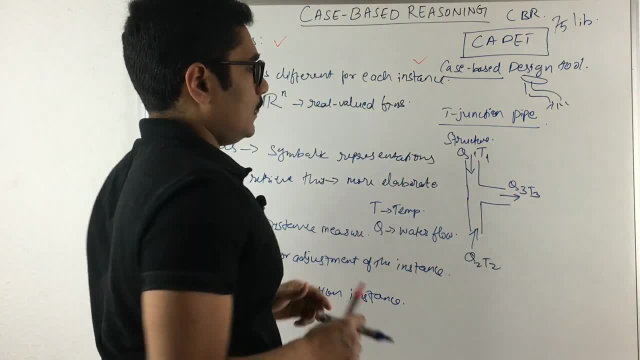 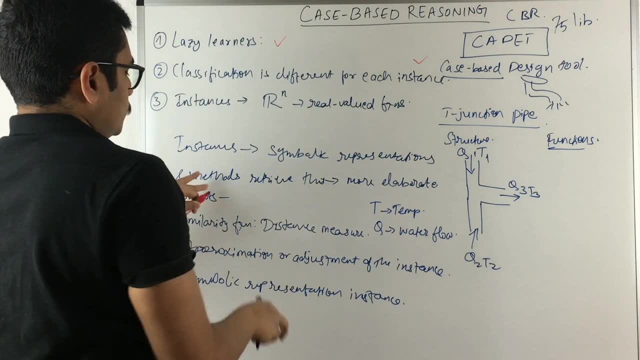 flow will be from this direction. So this is how the structure looks like. so the function if I want to depict. so we said that the functions are more elaborate, So methods retrieve this and it will be more elaborate. So say, you have q3 here. 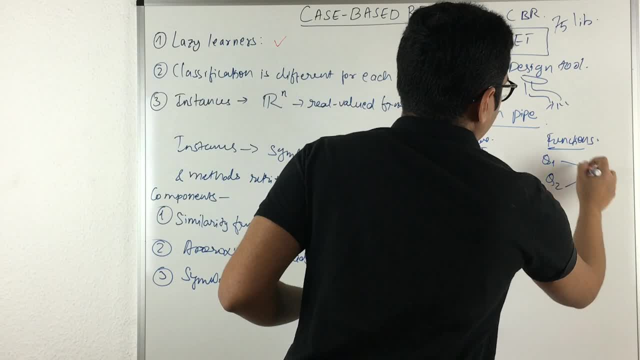 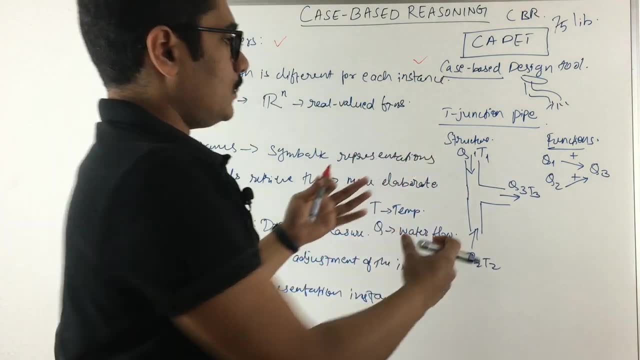 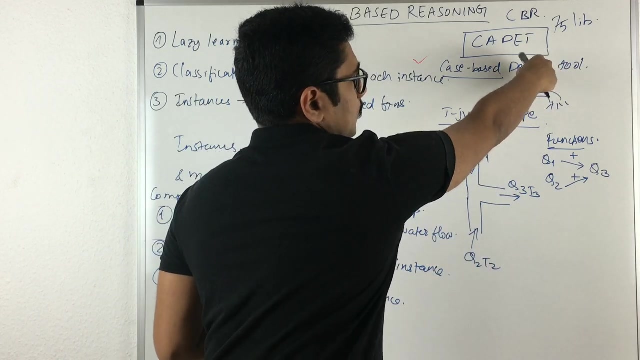 So since q3 comes from q1 and q2, you represent this by plus. so positive symbol represents that there is an increased water flow in that particular direction. And so if you just put this at the center, so if you just put these liver at the center, 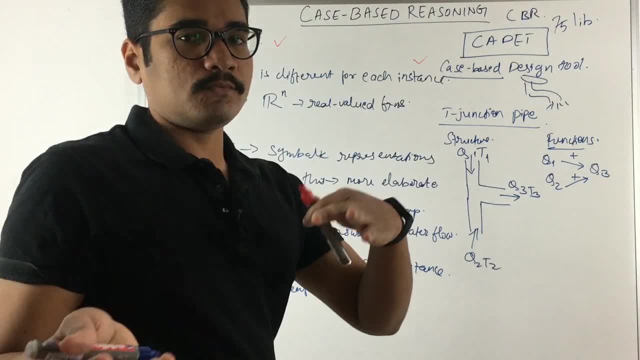 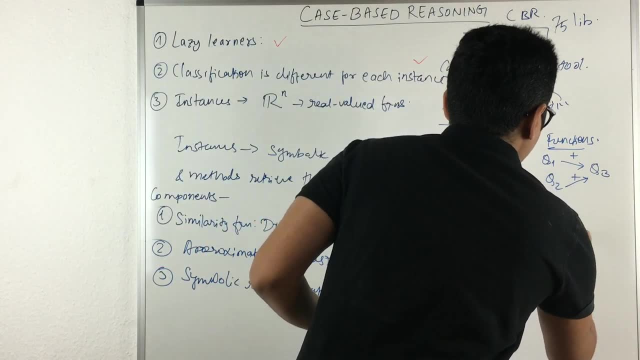 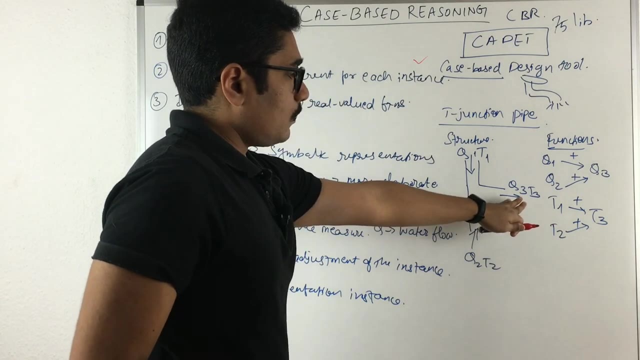 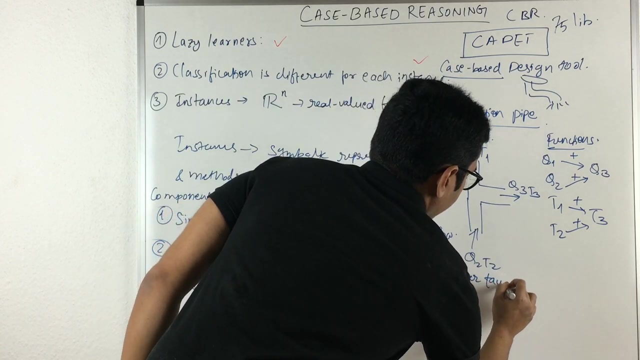 so then you will have a moderate water flow. That is basically a mixture of hot water and cold water, lukewarm kind of setup, and similarly the temperature is also like that. So you have t3 here, So you get a moderate temperature. So that's what this particular t-junction pipe represents. now our water faucet. 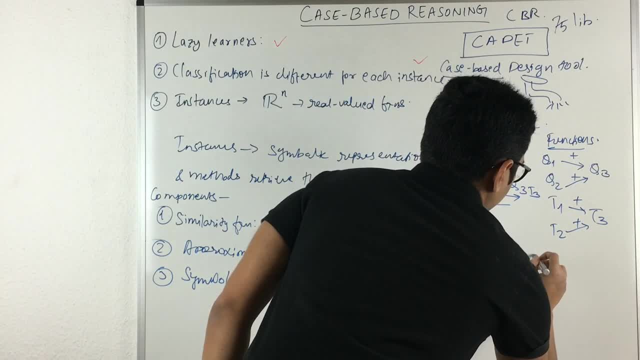 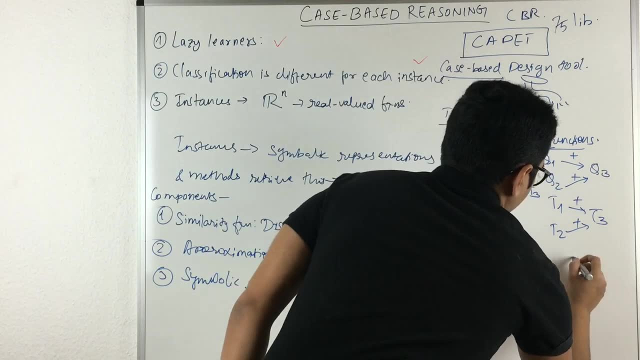 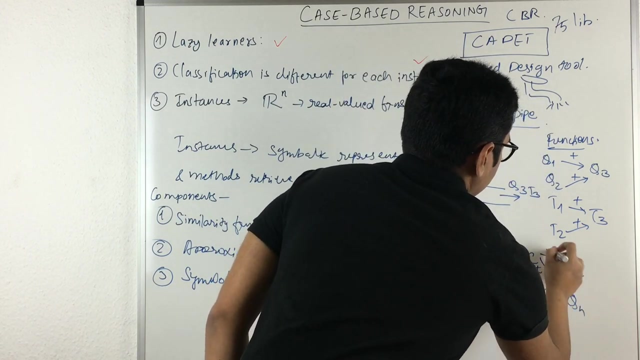 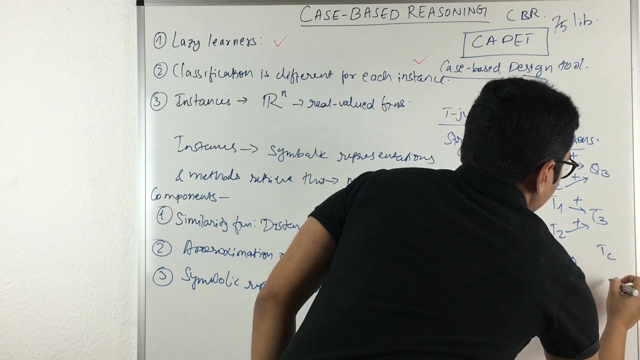 That is our problem. scenario is like, say, you have ct, That is, This is a control temperature, and you have control flow, is there. then you have qc and qh, so you basically provide some water flow from this directions and you have, say, cold temperature, mixed temperature and hot temperature. 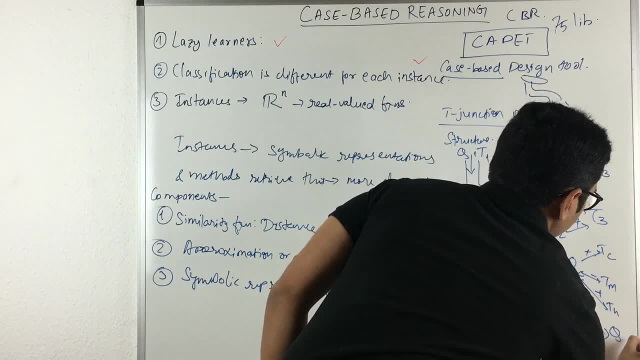 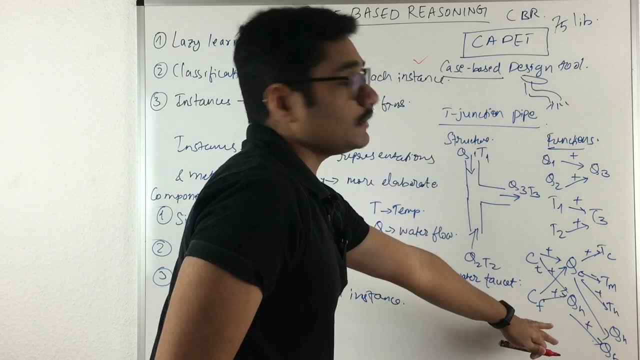 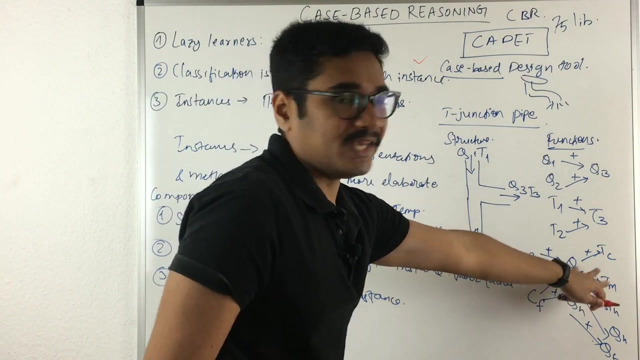 So then you design your system in this way, then qh, qt, So you basically provide some water flow from these directions and you have cold temperature, So you have a similar kind of setup like this. now you are given the function. So whenever the user says that I want my system to behave in this way, 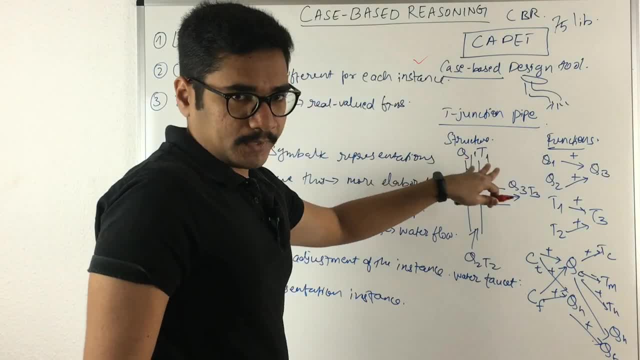 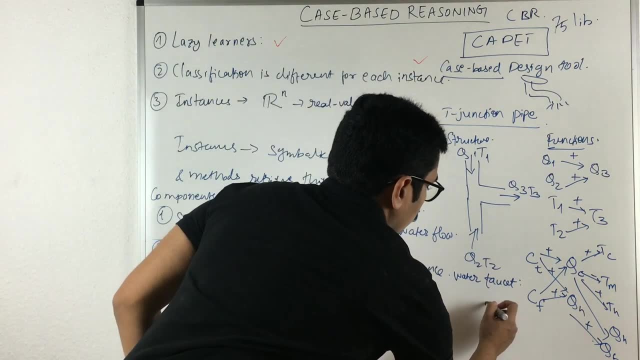 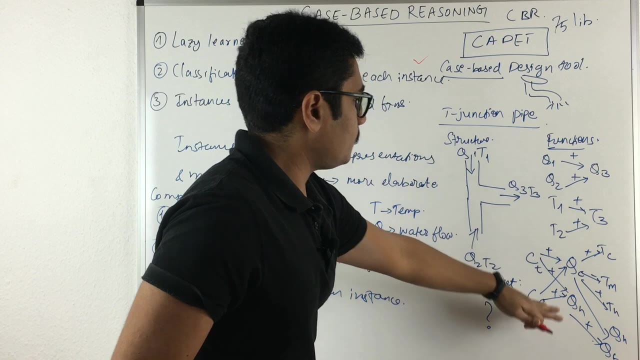 So this is more complicated as compared to the previous junction pipe. So, since this is the most similar setup that I have found in my case based reasoning system, now my problem statement is: how will I derive this structure? So what case based reasoning system does is? given this problem statement, and this is the 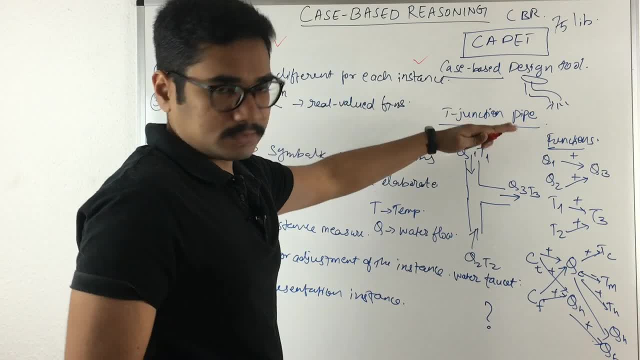 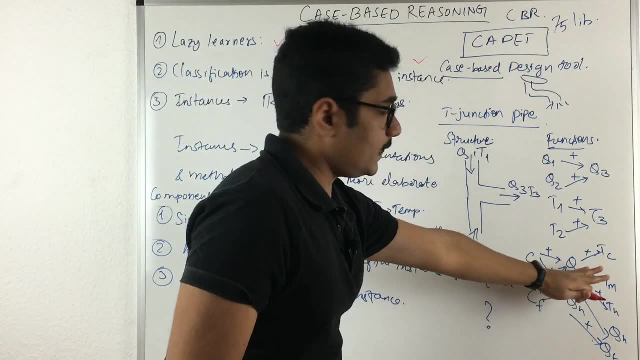 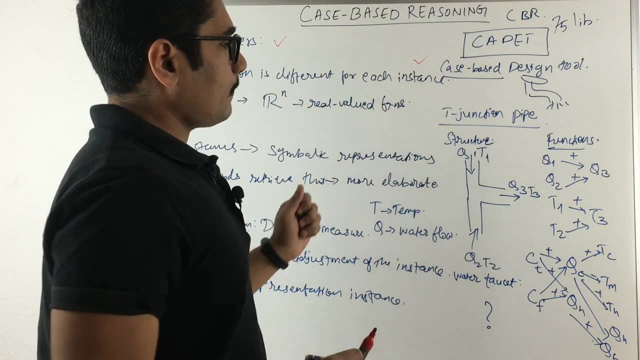 most matching similar use case that it has gone from its 75 libraries. It will provide some appropriate kind of structure in order to that. it will mimic this kind of particular setup. So this kind of case based reasoning systems are mainly used for some kind of problem deriving. 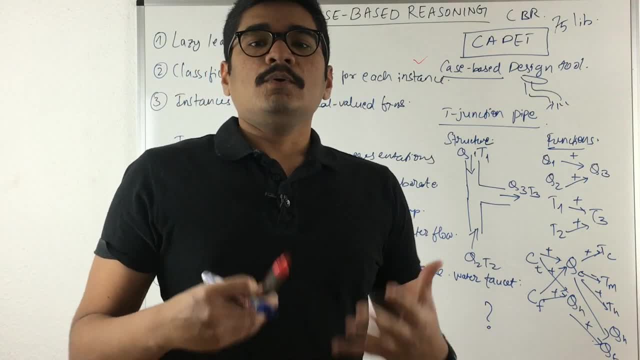 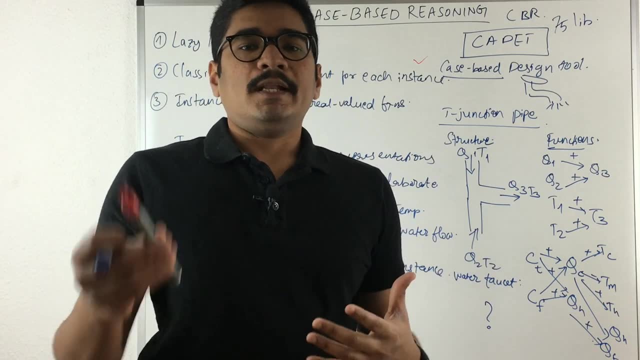 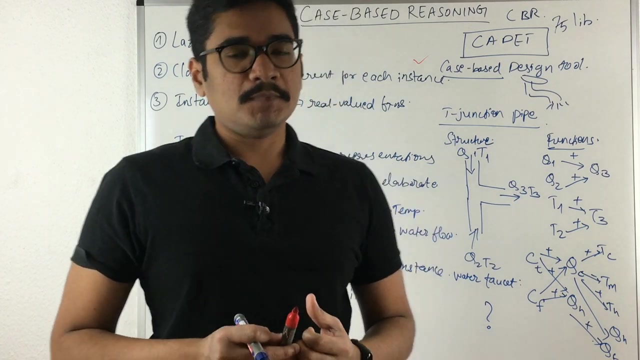 solutions like if you have some kind of patients Who can be prone to different diseases or some drug test disease. So based upon the previous health care records and Etc, they'll provide appropriate kind of solution to this. So well, that was all regarding the case based reasoning systems in machine learning. 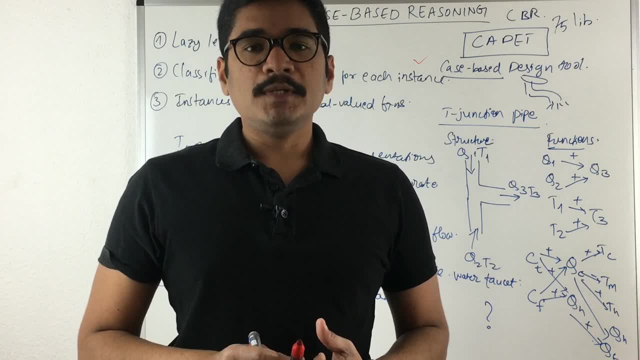 So hope you guys enjoyed this video. if you want to get educated on this video, please do like share comment and if you're new to this channel, please keep subscribing. Thank you very much for watching this video.